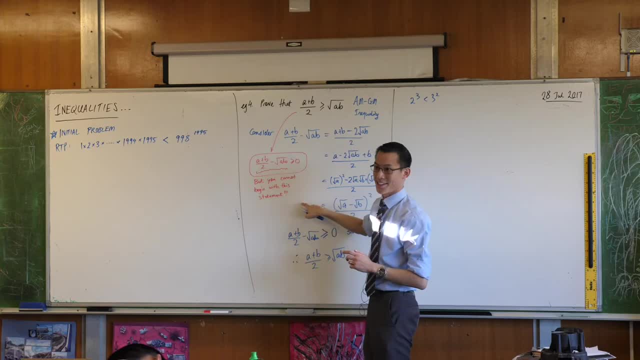 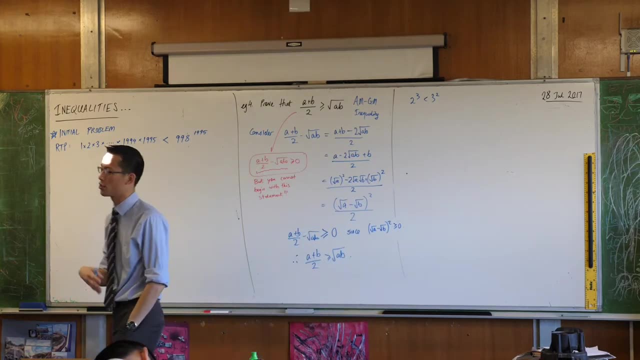 is greater than or equal to zero, And I've even written it here, just so that you can see what I mean. Here is why You cannot begin with this statement- and this is a very common error for people to make- because they do not understand the way mathematical deductive logic works. 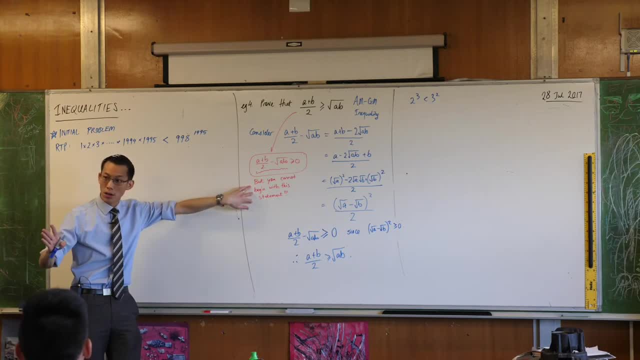 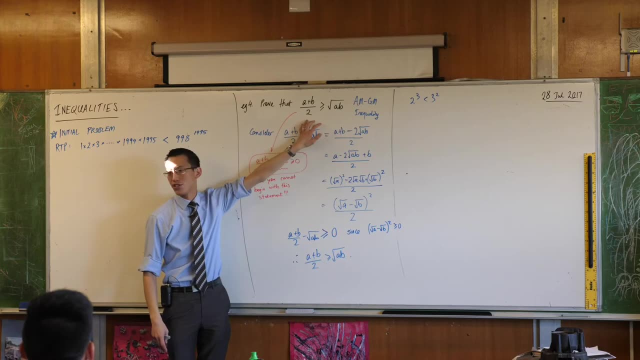 You can't make this statement as like your first line of working because you don't know that this is true. That's the point of the question. You're trying to prove that it's true. This is not an established fact that you can apply logic to, Unlike this being an established fact which you 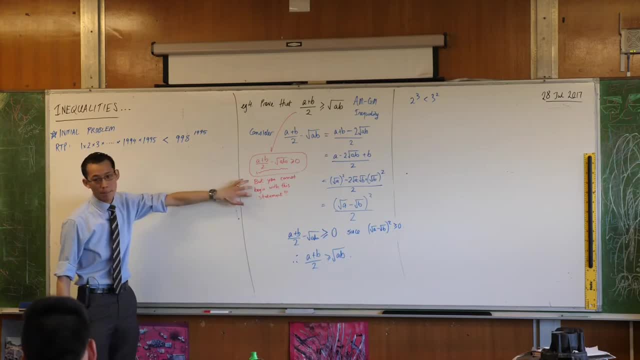 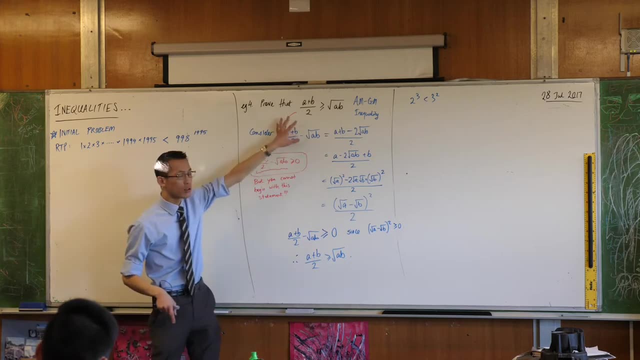 can apply logic to and then you can get to the answer. okay, So you can't begin with this statement. In fact, the first time that I actually write something like this is like right at the very end, after doing all of this algebraic legwork. okay, So when you see a 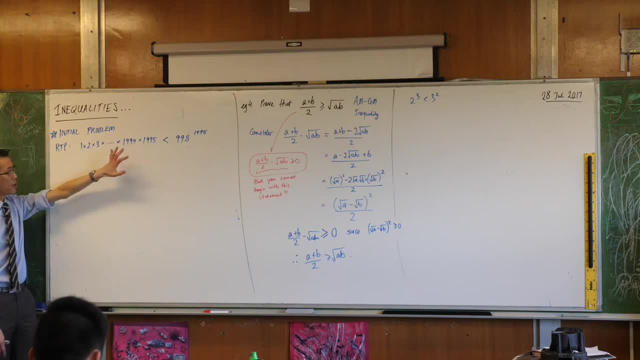 question gives you a result like say this okay. You can't say, oh look, here's a result. I'm now going to start doing some stuff on the left and right hand side of this, as if this were true. 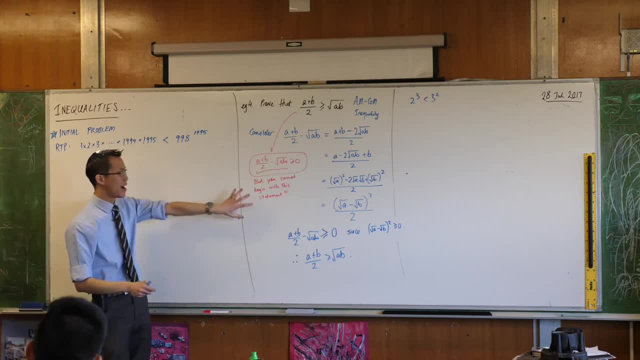 because you do not know that it's true yet, okay, So that's why I put this in big red letters. You can't begin with this. You can think it, but you can't get to it till the end. okay, Here's the actual question. 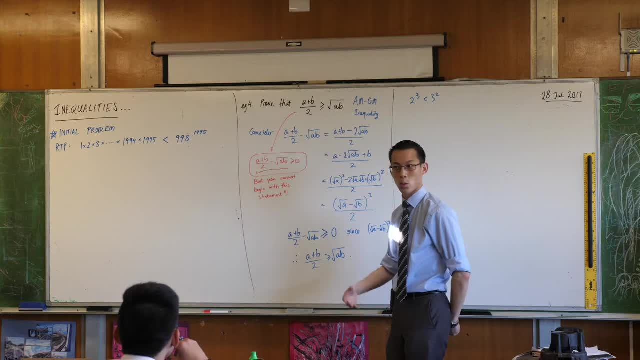 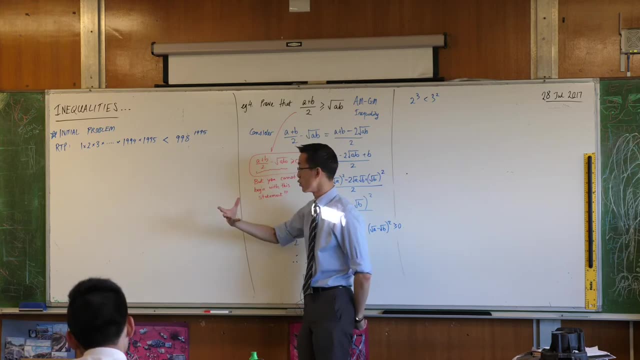 I've written down RTP here, which is just my abbreviation for required to prove, just to highlight the fact that I just said I don't know that this is true yet. Me writing it down doesn't mean I think it's true. Me writing it down means: okay, I need to get this down. so 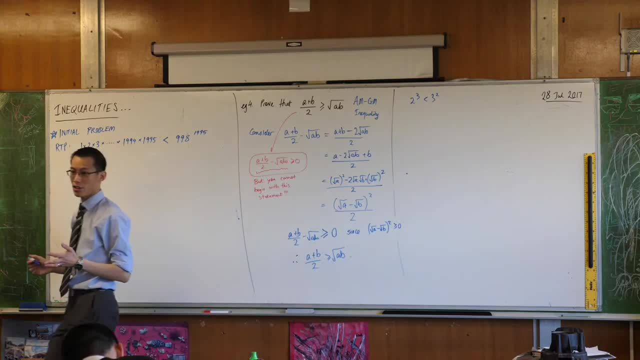 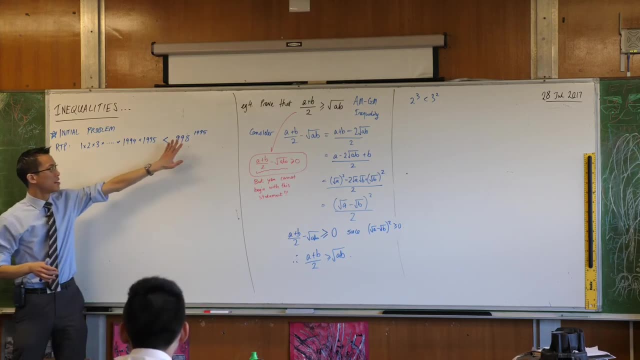 that I can apply some logic to it. So what strategies shall I attempt? Just like in earlier problems, like, say, that one, the first thing I'm going to do is try and pare this down to size This number here. I think it's one of those numbers that make your calculator break, right? 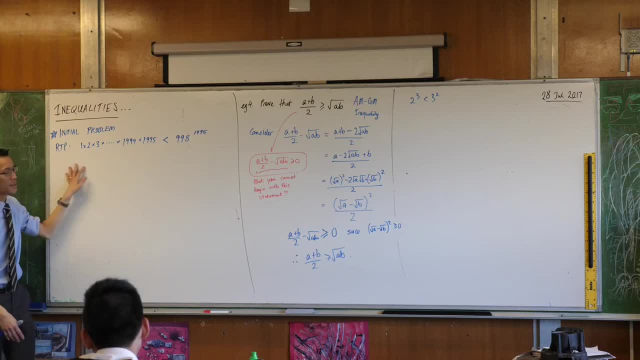 I don't know what to do with this, okay, So therefore, I'm just going to think about this guy over here for a little while. I'm just going to consider the left-hand side. okay, The left-hand side reminds me a lot of the work we did with series and sequences. 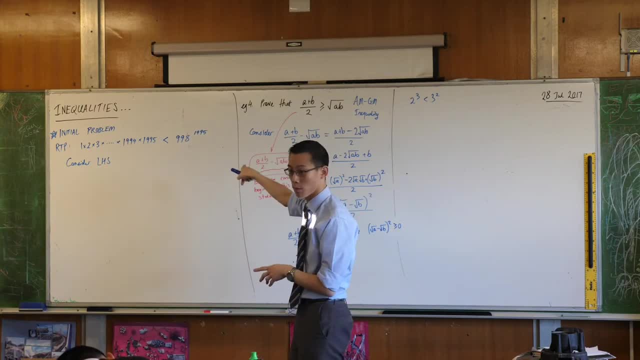 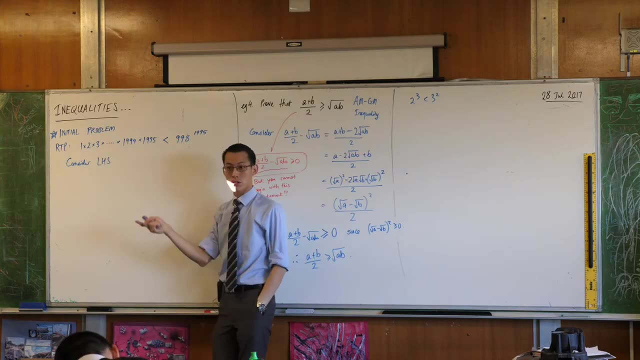 It's not a series or a sequence. You know, adding things up, you're multiplying them, but I can apply some logic that I used back there. for instance, This is a very, very logical set of numbers, right With the order. there you can see, you can predict exactly what's going to be there and in fact you can use itoredically. 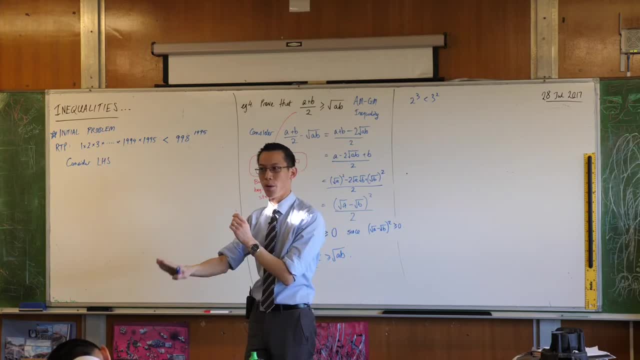 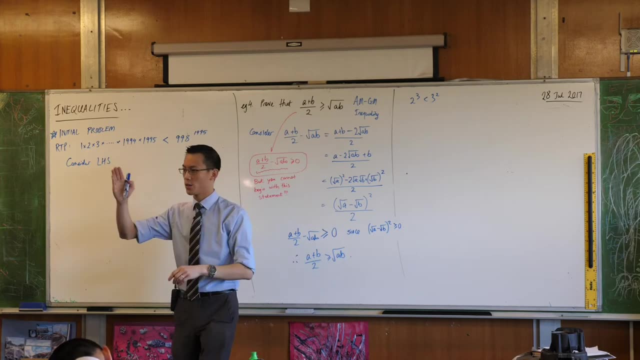 trick that we learnt from little boy Gauss when he was asked to add up the numbers 1 to 100.. Do you remember what he did? Sorry, 1 to 50? 1 to 100. No, it was 1 to 100. He. 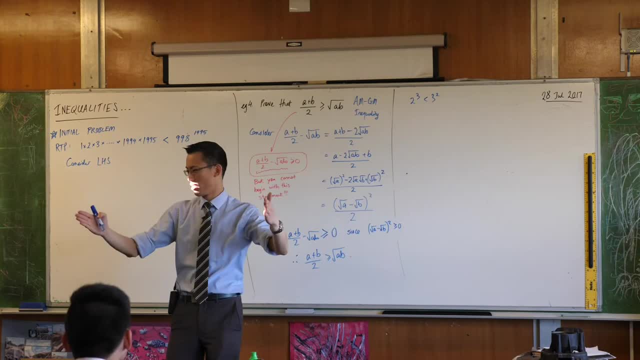 was like 1 plus 2 plus 3 plus 4, all the way up to 99, 100.. Doing them in order, that's like a chimp's way of doing things. That'll take me forever. He noticed a pattern, if you. 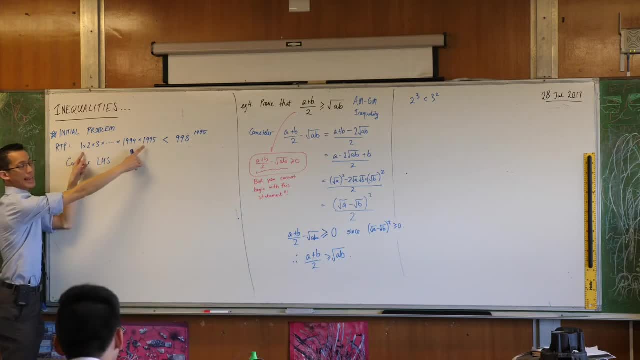 look at it from both ends. He said: if you pair up numbers, if you pair up numbers, if you pair up numbers like- so I'm even going to write it- I should be able to notice there's some logic here that I can take advantage of. Now, when you pair in this way, think: 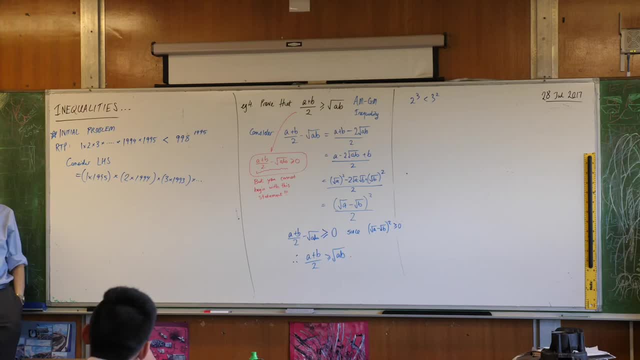 carefully. what will you get to? What will be in the middle? The numbers are a little bit large so it's kind of tricky. Think to an example that you know It's easier. Sorry, There's an odd number of terms here. Do you agree An odd number? 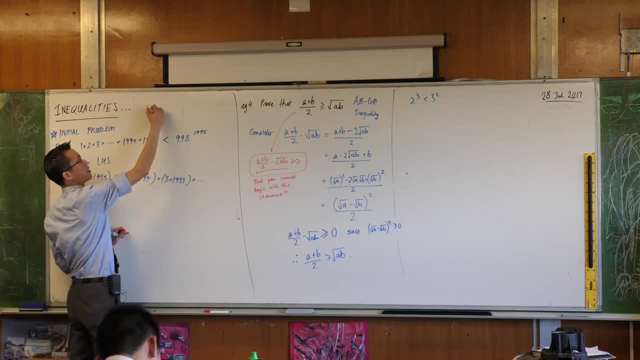 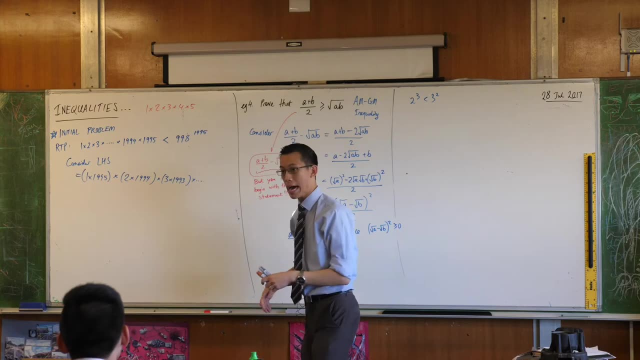 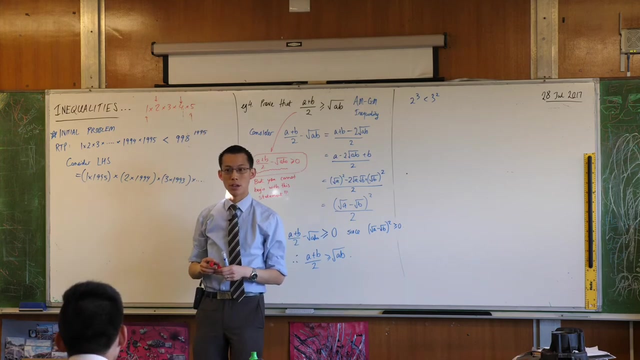 of terms. So I'm going to think of a simple example with an odd number of terms. How about this? So if I had that, if that was my product right and I did my pairing thing, you'd pair up these guys, then you'd pair up these guys and then you'd end up with a middle term. 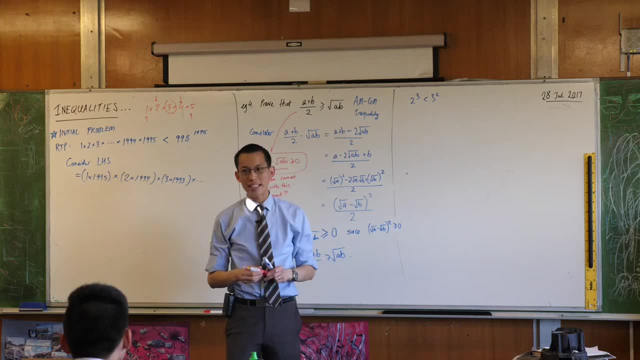 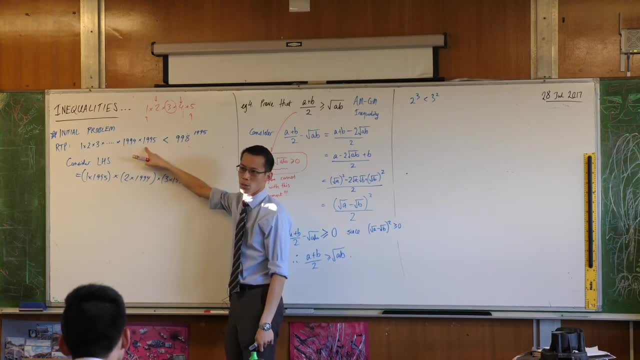 could I go directly there? if I had like an obscene number of terms, What would I do to get to 3 quickly? Okay, so one of the ways- and there's lots of different ways- is I could add 1 to this to turn it into an even number- 6, and then divide by 2, because I'm halving. 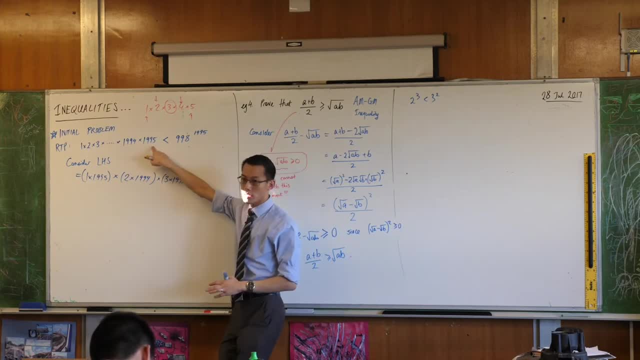 aren't I? Okay, Since everything is paired up. So if I add 1 to this, that gives me 1,996.. When you divide that by 2, you get 998.. That's suspicious, right Okay. now 998 will be the very, very last term. It's on its own, It doesn't pair. 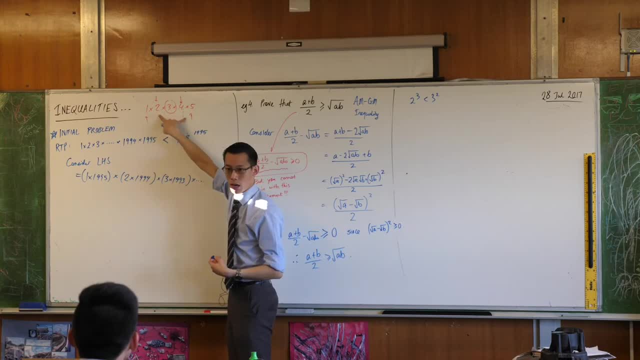 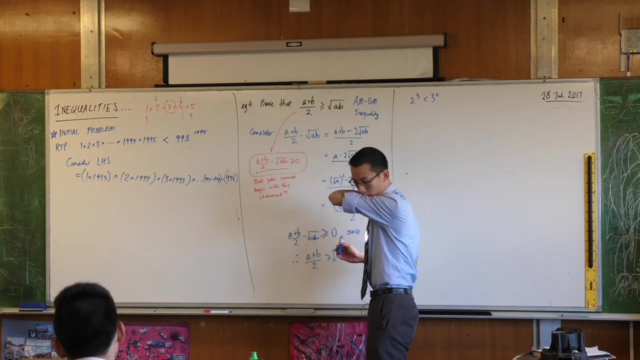 with anyone. So therefore, by that logic, what are the two on either side, What are the numbers that are going to appear before that? One will be smaller and the other one will be bigger. Okay, good. So what we've done is we've broken up this long product into. 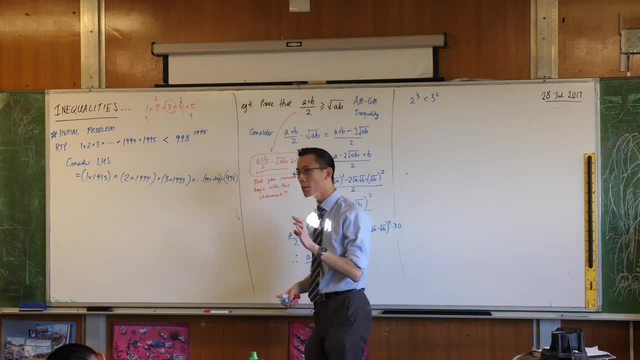 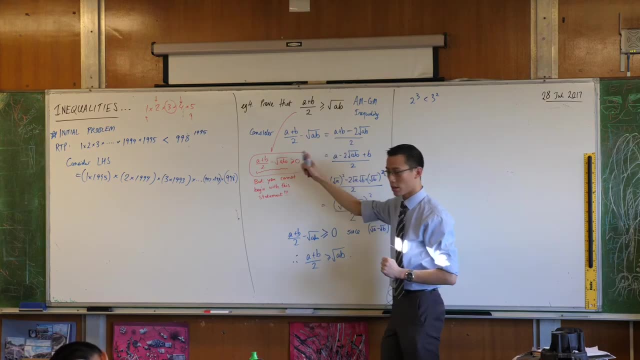 a bunch of pairs So that are easier to deal with. Okay, now I'm going to use some logic from the immediately previous example that I showed you. Okay, have a look at this. This is telling us here. it's telling us here that the square root of a product- square root of a product- is: 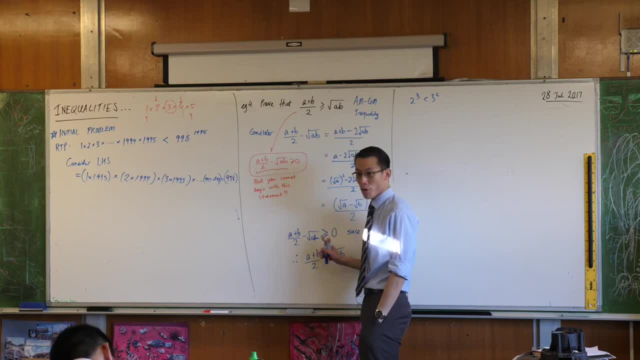 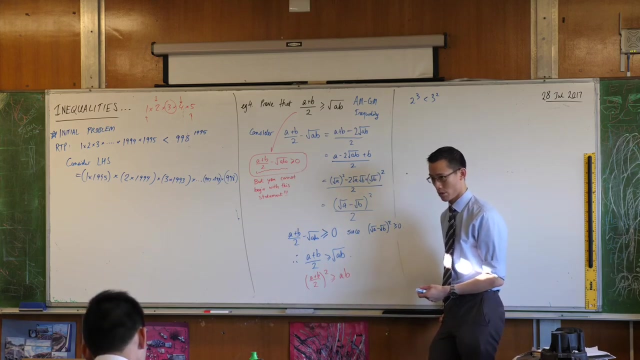 always less than or equal to this thing over here. Okay, well, if you go back again, another example you can see from this, I could square both sides like that And that would be less than this, Do you agree? That's okay right Now. how does this in? 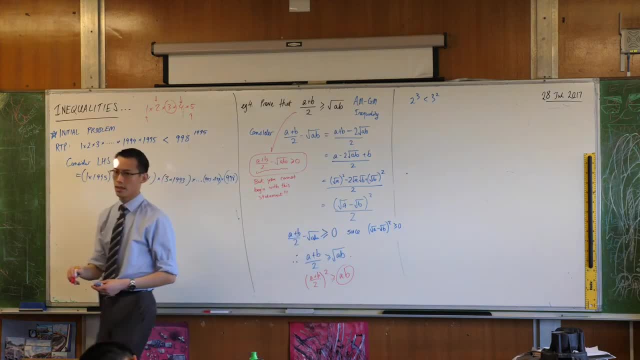 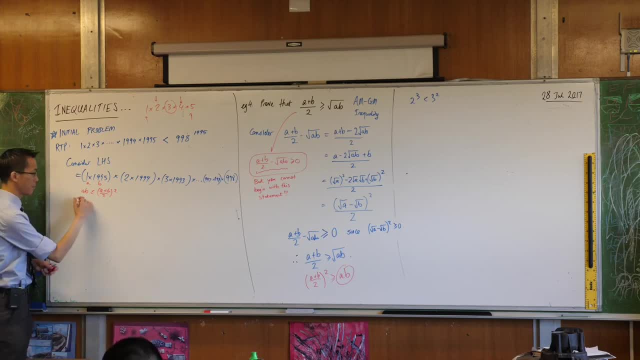 in this case, for this a and this b, 1 times 1, 1, 9, 5.. It's less than or equal to what. Have a look, We just did this, didn't we Like? we literally did exactly this. This is: 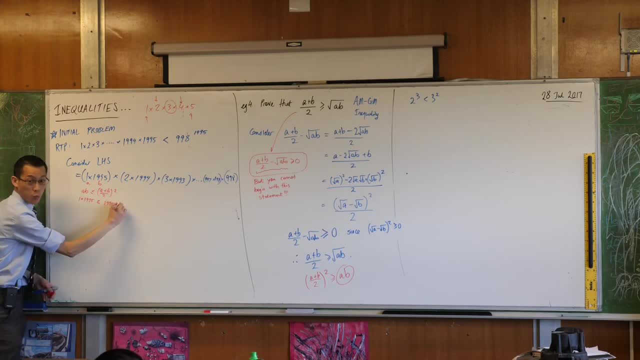 Tina's suggestion. I took a number, I added 1, and I divided it by 2.. Yes, So this little product here, this pair, is going to be less than or equal to. that is 998.. How's your brain? 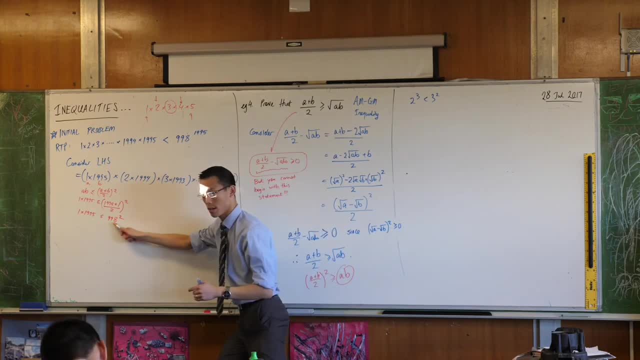 going. Do you see what I'm trying to do here And do you see how this does connect us to this? Ooh, I've got powers of 998.. That looks helpful. When you look at the next one over, it doesn't take you long to realize that having this, 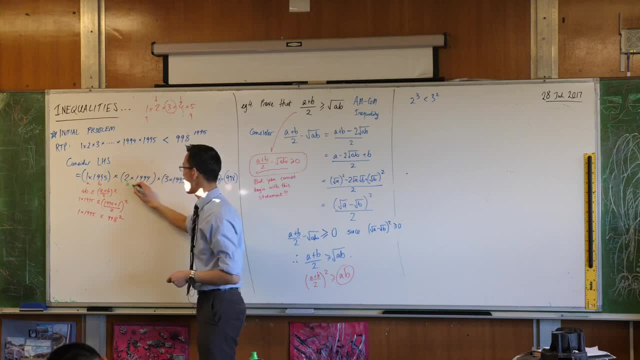 pairing up thing is super advantageous Because, look, here's a new a, and here's a new a is a new b, And so this ab is less than da-da-da. is all still true, right? So I can say I. 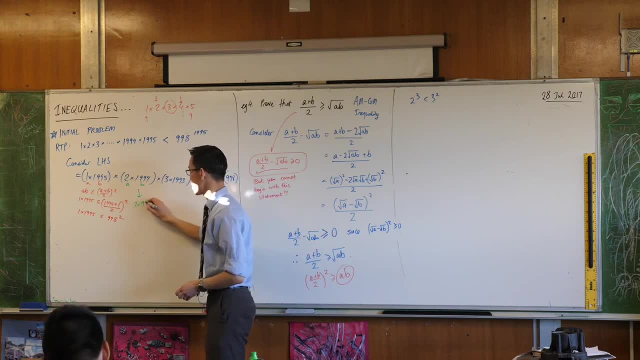 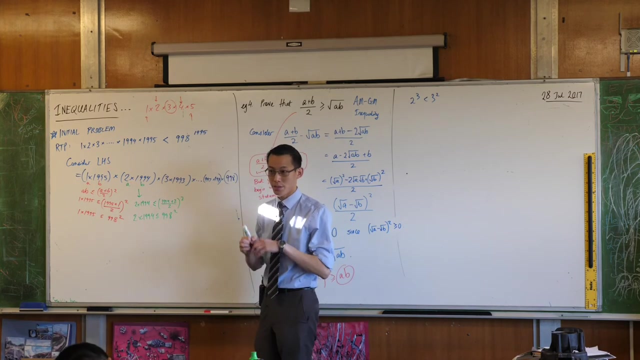 can skip straight to this line that 2 times 1,994 is less than or equal to 1,994 plus 2 on 2 squared. But again, because you've formed these pairs in this way, this is still 998 squared, Do you agree? Okay, So what I'm going to do is remember: inequalities are: 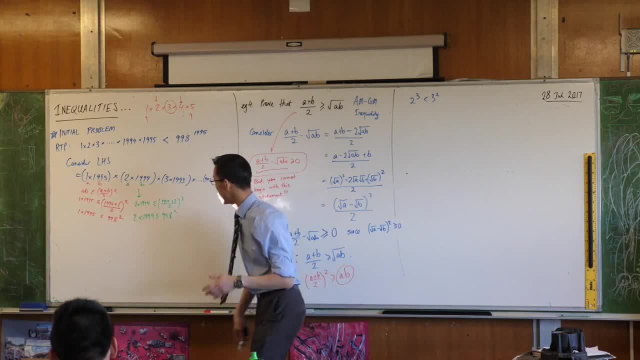 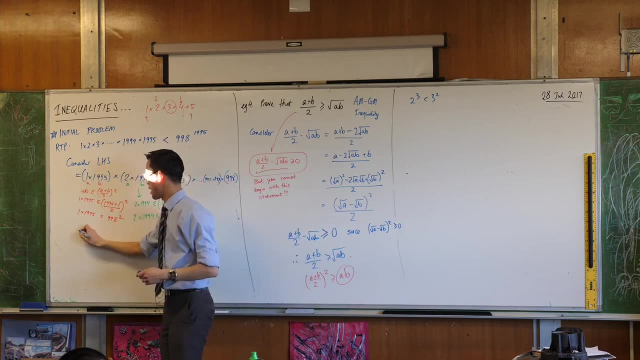 a little bit different. Nope, that's the color I want. A little bit different to equations. I can swap all of these things out. I can swap all of these things out for something that is bigger. Okay, So I've still got my left-hand side over here, But what I'm going. 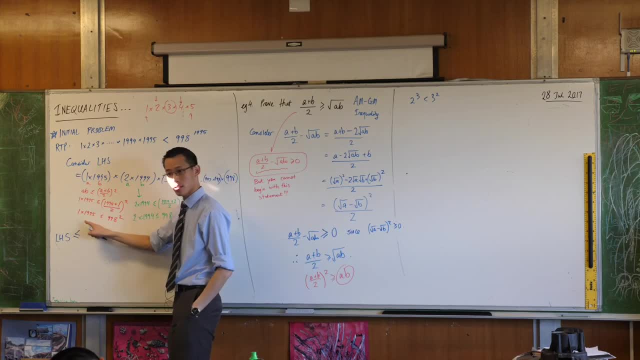 to do is see how 998 squared is bigger than this. Well, if I swap this for 998 squared, then what I've got over here will be bigger than what I started with. Does that make sense? So I'm swapping out a number for something. 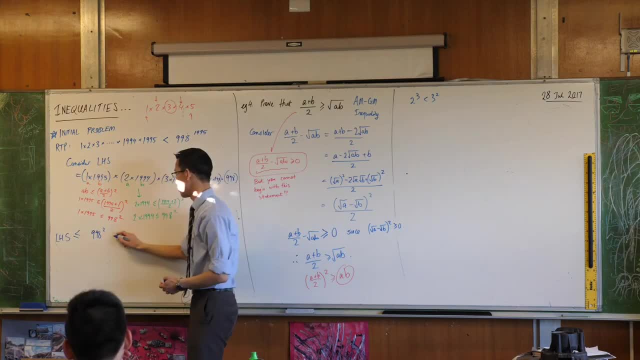 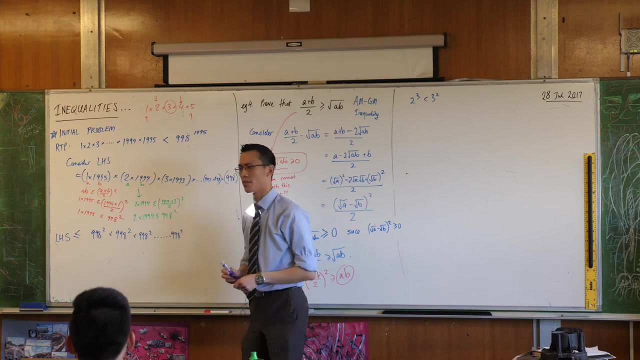 bigger. I'm going to swap out this number for something bigger as well, Like so, And this will also be that. Now, this is going to keep on going. I've got a lot of pairs, don't I? How many pairs do I have? 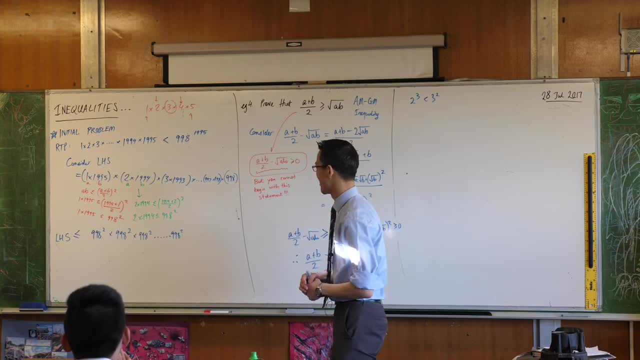 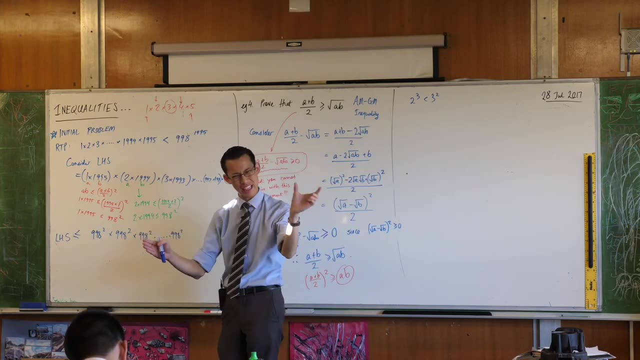 If you think back to when we were doing sequence and series. when you've got an infinite series or sequence, we go dot, dot, dot and it just goes on forever. But we know when it's finite. that's why we put the n term on right, Which is why I put this guy here. That's the last. 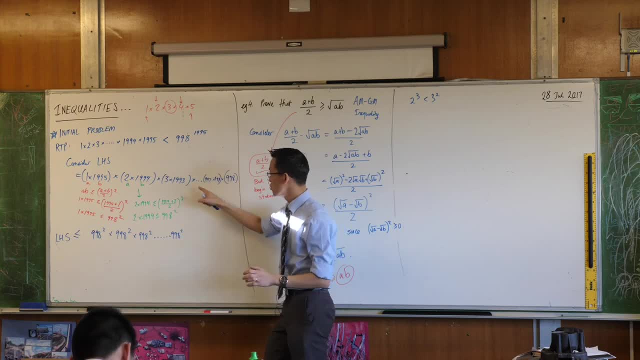 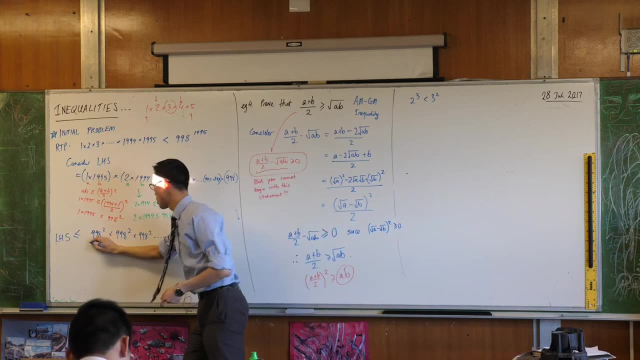 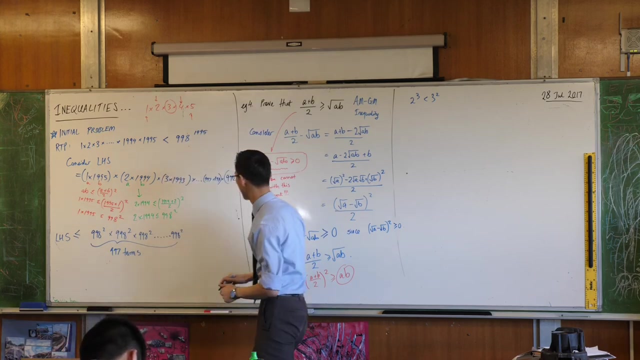 term in this bunch of products. So you can see it goes 1,, 2,, 3,, 4,, 5,, 6,, all the way up to: So there are 997 of these. Does that make sense? I'll really quickly finish because I know you've got to go to a roll call And then 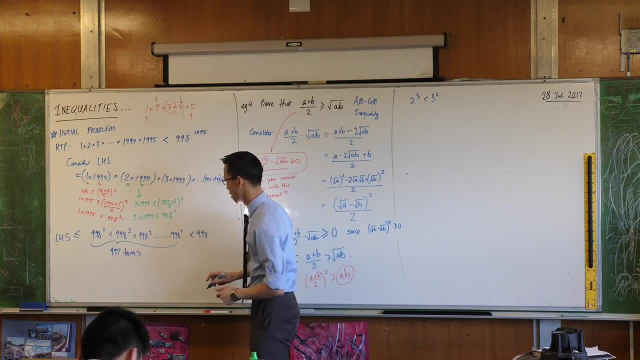 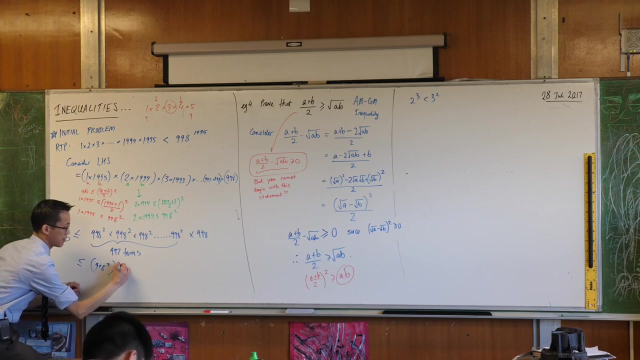 there's this hanger on the end, the ultimate third wheel, except he's the 998th wheel. So there you go. So now I'm almost there. I'm so close. Just use some index laws for me. here I'm multiplying 997 times. So this is this, multiplied by itself 997 times, And